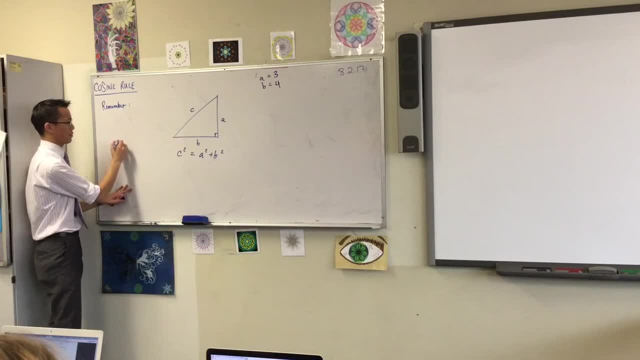 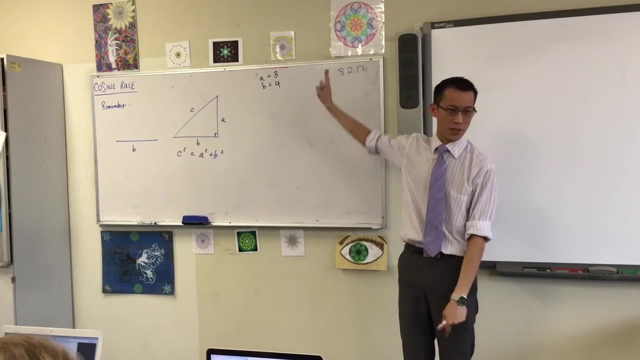 My B. I'm calling that 4.. Whatever your B is, I want you to make another base of a triangle that's the same length, whatever that happens to be. Then what I want you to do is Is to get another side that's going to be the same length as A, whatever your A was. 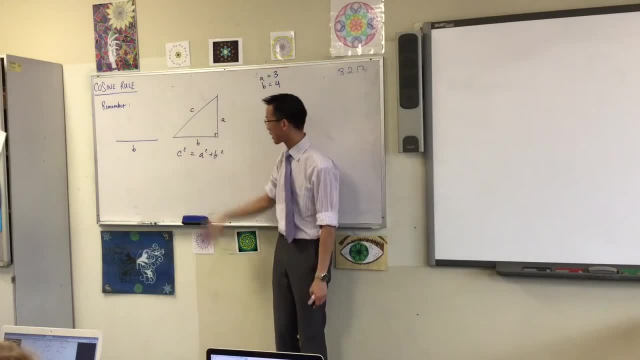 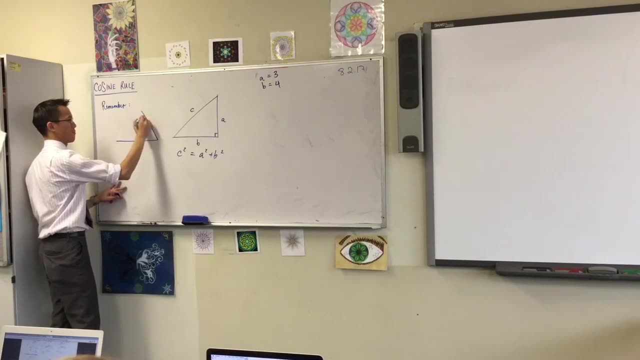 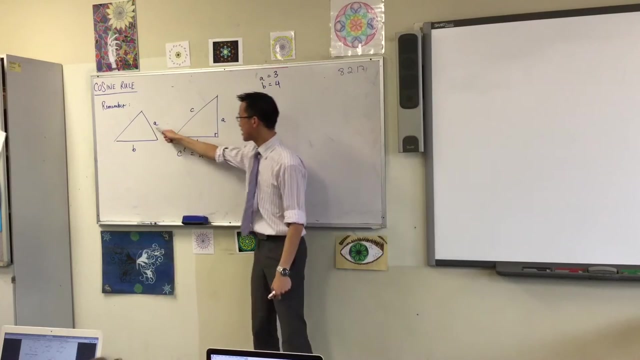 But this time, instead of going straight up, straight up, I want you to lean it over a little bit, So it's not a right angle. So I'm going to draw mine like this: Okay now, it's really important on your diagram that this A and this A are the same, this B and this B are the same. 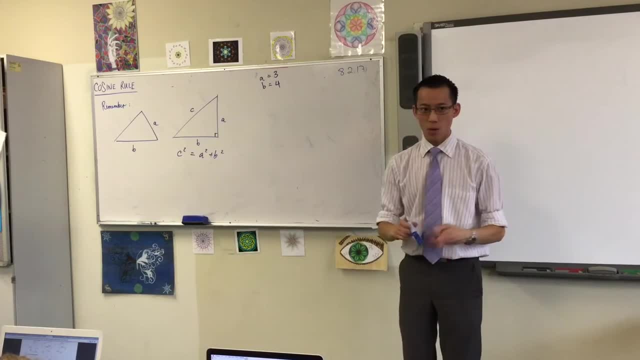 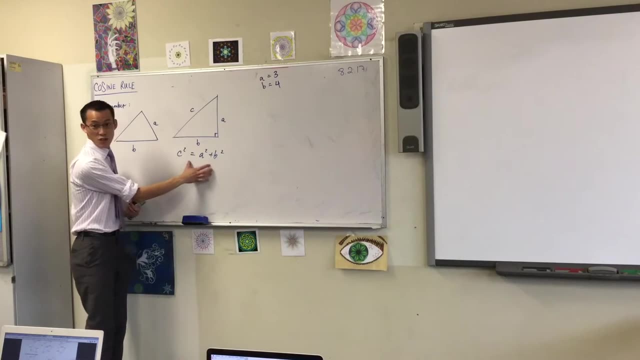 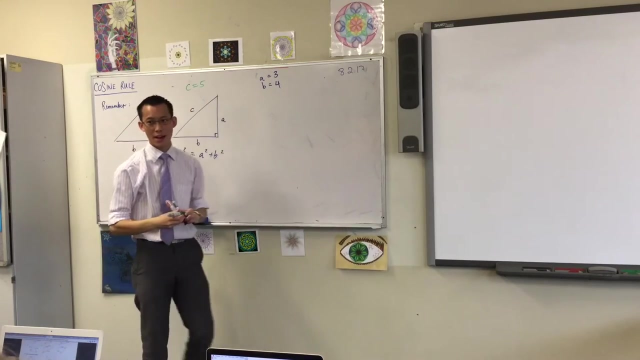 Okay, now, Once you've done that, I want you to have a look, and we might need some colors for this one In your original triangle, this triangle that you started with. now, I want you to measure C Right. for me, I would have had C equals 5.. Okay, because it's right angled: 3 squared, 4 squared, 5 squared. 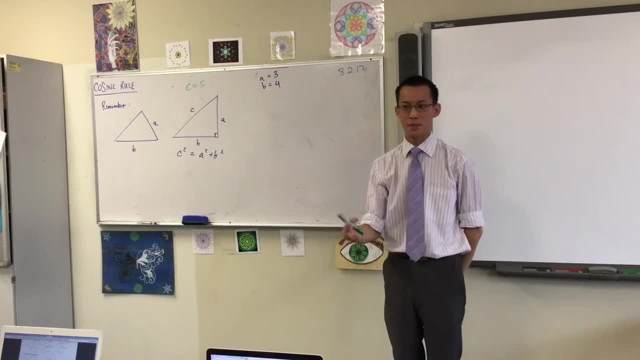 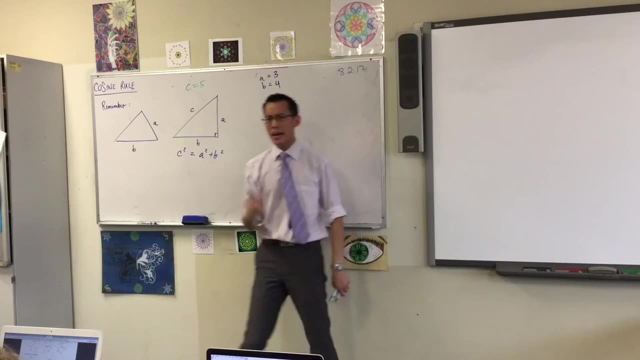 Okay, I want you to measure your own one. Okay, whatever happens to be 4.5 centimeters, 8.7, whatever it is, and I want you to write it just above here. Now, this new triangle you've made, it's still got the same A, still got the same B. 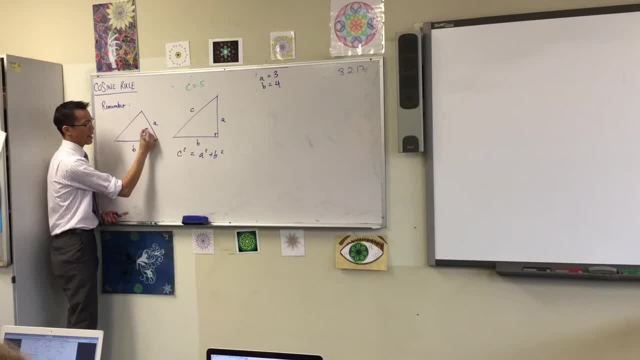 But now it has, and I'd love you to write this in as the case. Now it has an acute angle in there. instead of 90 degrees, It's leaning over. Now, what I want you to notice is What's happened to C. I want you to measure it on your own diagram. 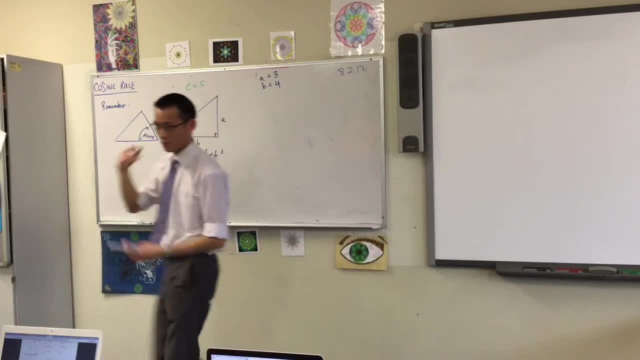 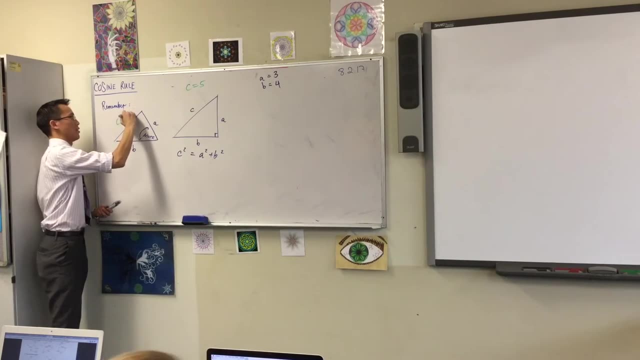 Okay, I'm just going to fashion a C, because I've actually drawn this out on my own piece of paper, But I can't, you know, it's not big enough. Okay, the C that I got for this triangle over here Was about 4.3.. Now I want you to think: 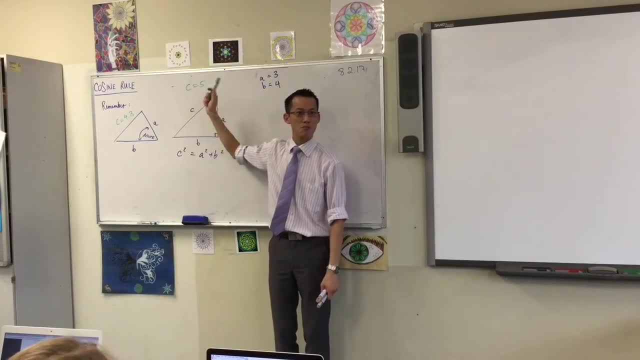 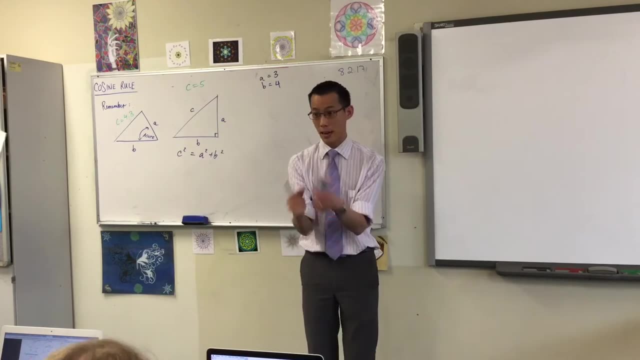 Have a look at whatever your C is. Do you notice you must have whatever you started with. you must have made a new C That was smaller. Did you notice that? Have you measured them? I don't know how much smaller, but it has to be a little bit smaller. Can you see why that is? 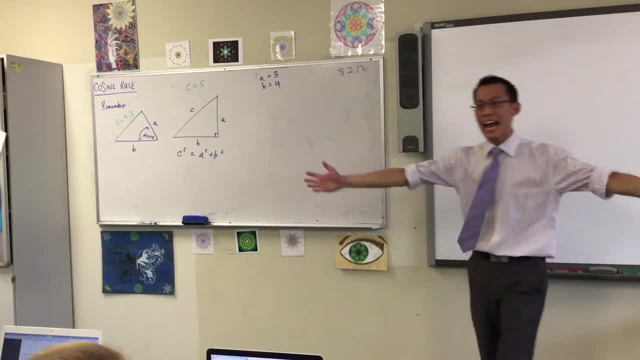 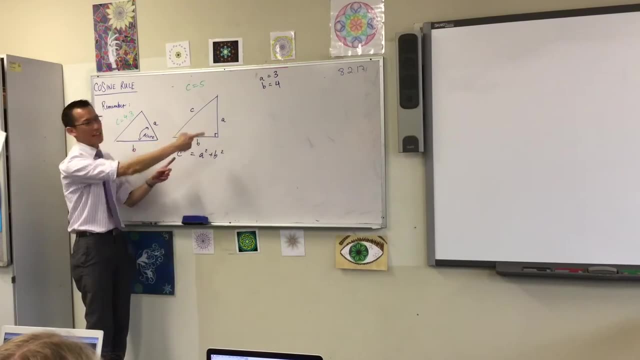 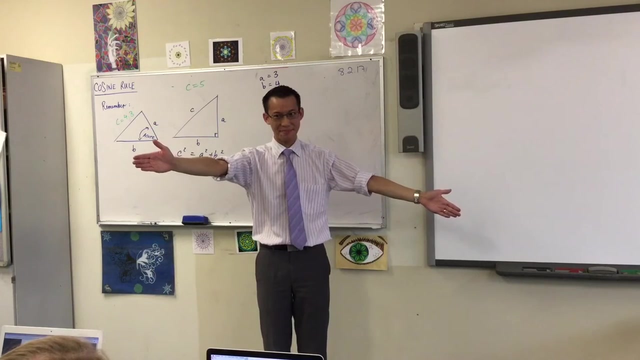 Do you remember It had to do with this thing? Do you remember that? Okay, I want you to think: A and B are your arms that for some weird reason, are not the same length. Okay, when you take that angle between the arms, This is how we're doing: half A, B, sin C, right? 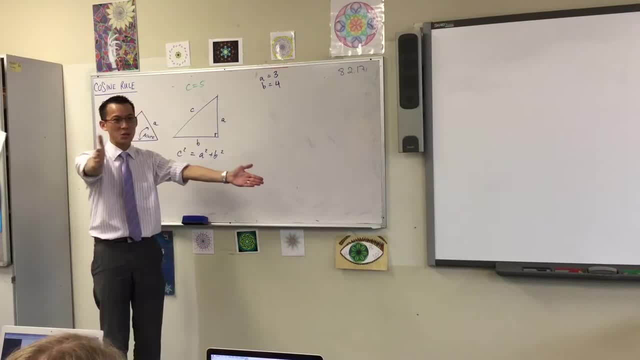 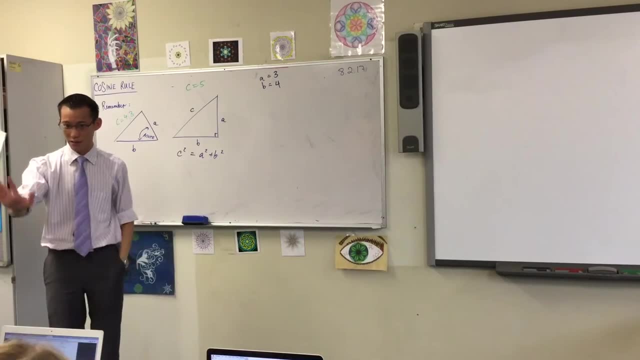 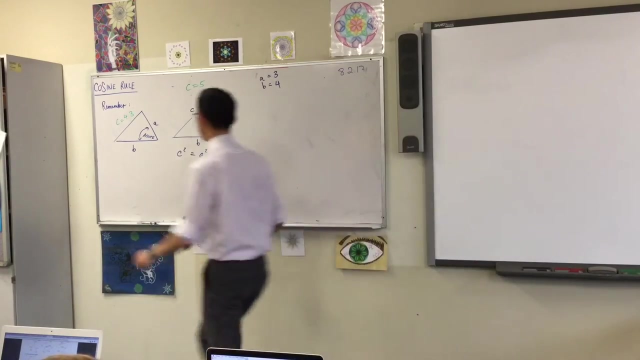 When you take the angle between your arms and you make the angle smaller, what happens to that length connecting your hands? It also gets smaller. It has to. there's no choice. So C gets smaller with the angle. Okay, stay with me. stay with me. 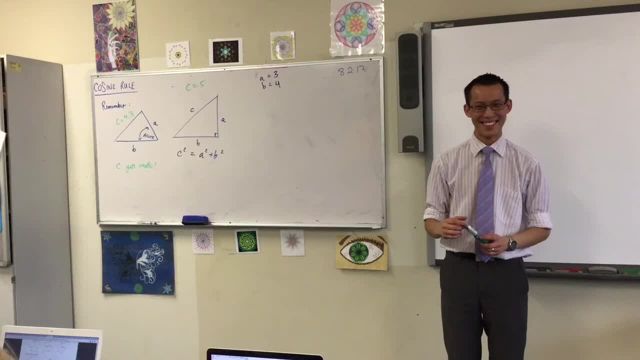 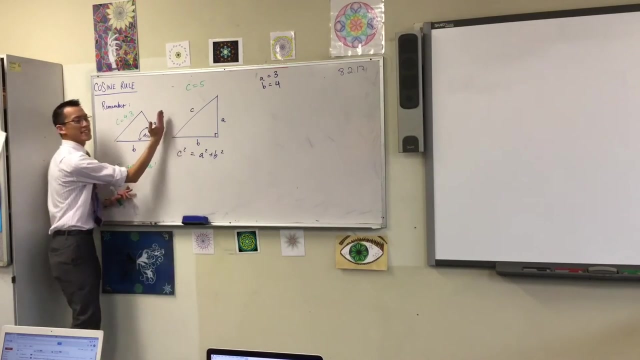 Just waiting for everyone's attention. We went from a right-angled triangle to an acute triangle. We noticed that C got smaller. What do you think I'm going to do? going this way, I'm going to make the angle larger. Instead of leaning A over to the left, I'm going to lean it to the right. 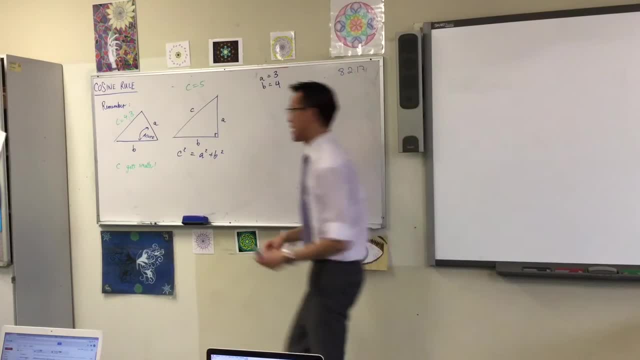 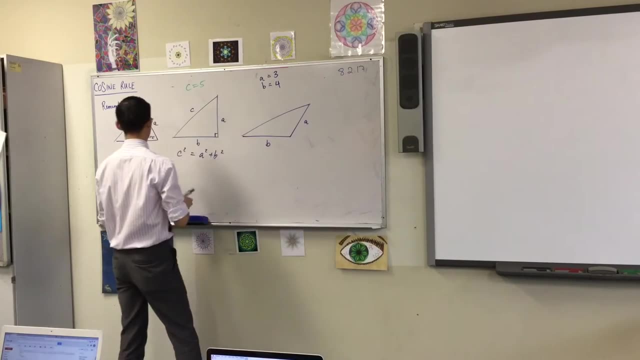 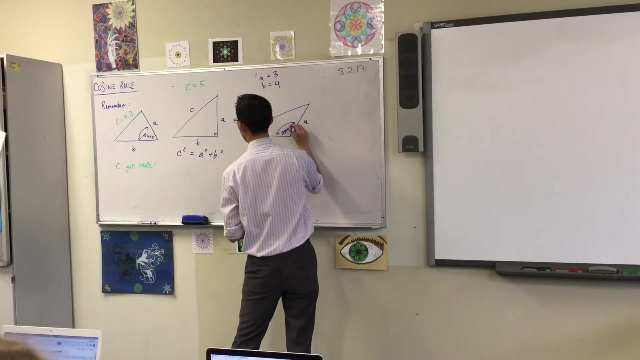 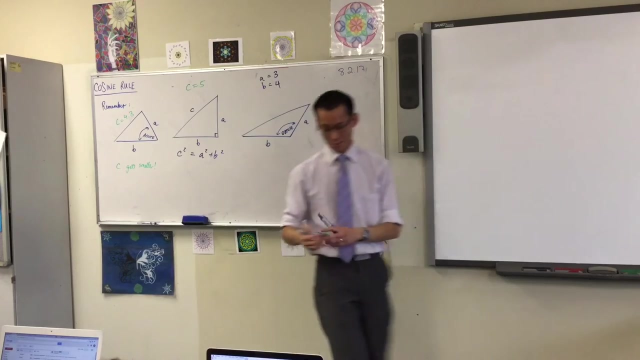 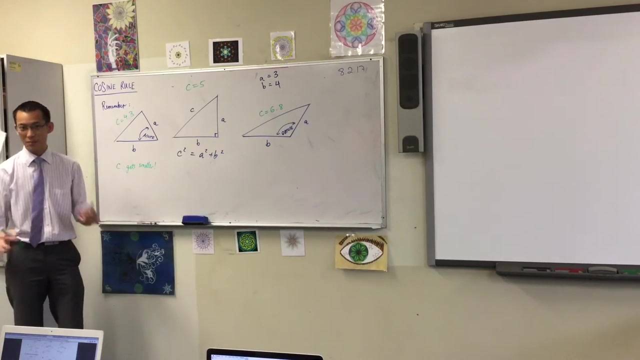 So go ahead and do that. Remember A and B have to be the same. Okay, now again. when I prepared earlier, the C that I got was 6.8.. And again you'll have something different. but you notice, the size has to go in one direction. 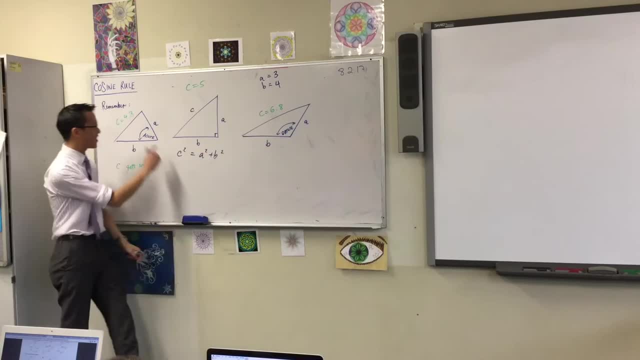 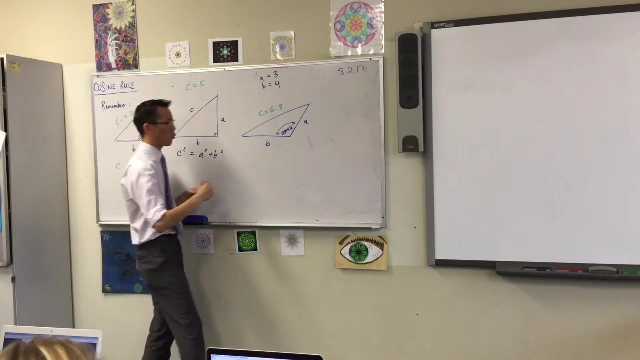 Boy bands. The angles get bigger. right, That angle in the corner goes from acute to 90 degrees to obtuse And in the same way this side C also gets bigger: 4.385 and then 6.8.. So with a bigger angle you get a bigger version of the hypotenuse. 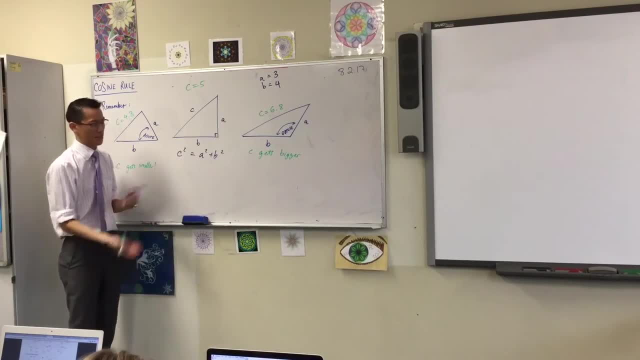 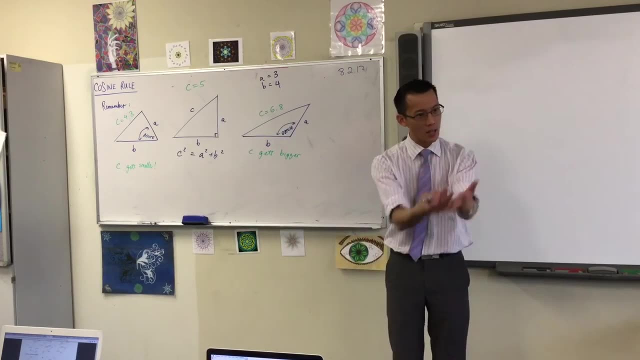 I call it a version of the hypotenuse, because of course these two don't have hypotenuses. There's no writing. Now, here's the beautiful thing. The cosine rule says it answers the question. well, if it gets smaller, how much? 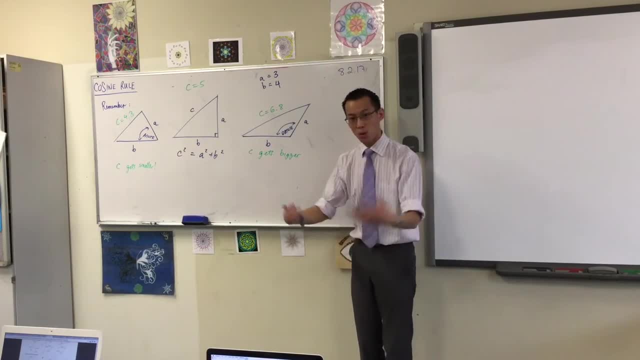 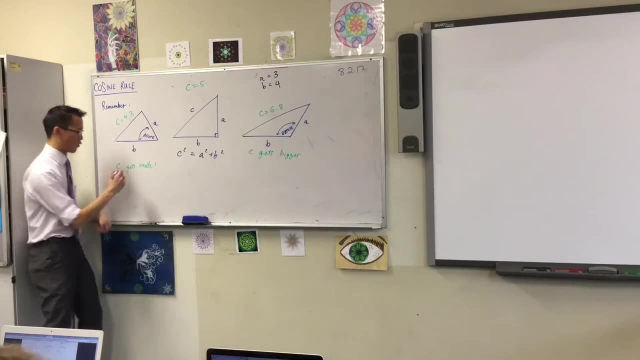 And if it gets bigger, how much, How much, How much, And it balls it together. It balls it together in one really elegant rule. Here's the way it works. You start with Pythagoras. Write this down again for me. 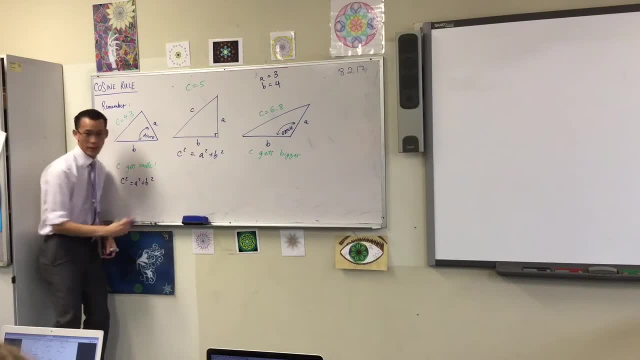 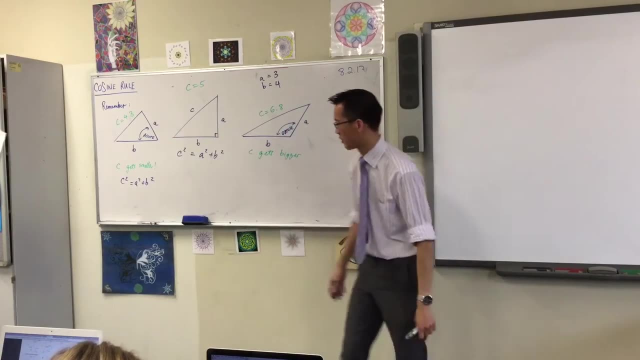 C squared equals A squared plus B squared. That's where it begins, But- and there's a fancy proof for this that I'm not showing you because it takes some time and it's actually not necessary for us- They adjusted a little bit. 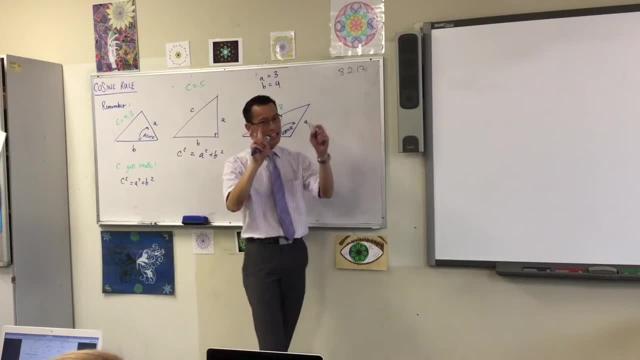 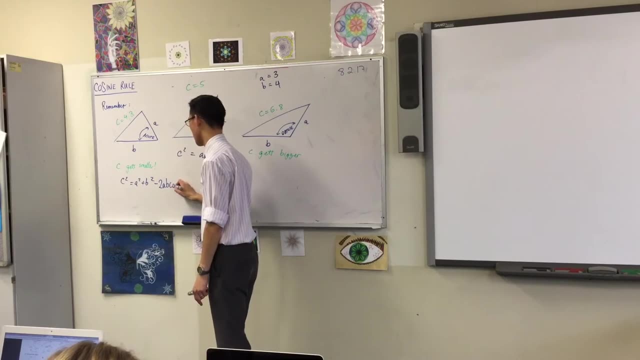 You see how I got smaller by a tiny bit. That tiny bit can be worked out with cosine. This is what it is: Minus 2A, Minus 2A. Minus 2A plus B, minus C. okay. 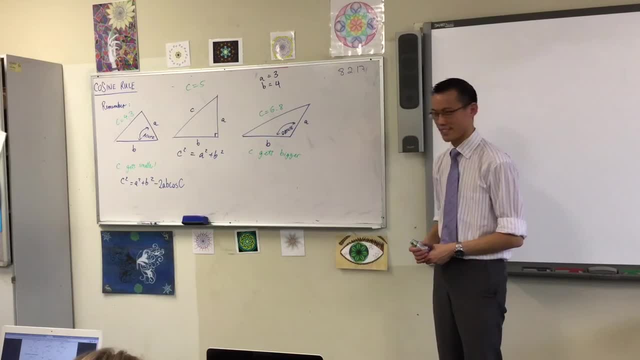 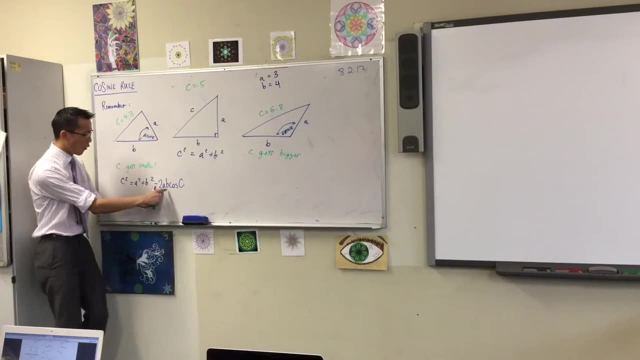 Minus 2A minus C. It's a little bit like that half AB sine C thing, but slightly different. okay, Again, this is on your formula sheet. The important thing I want you to notice is where the letters are, because remember we said those are important. 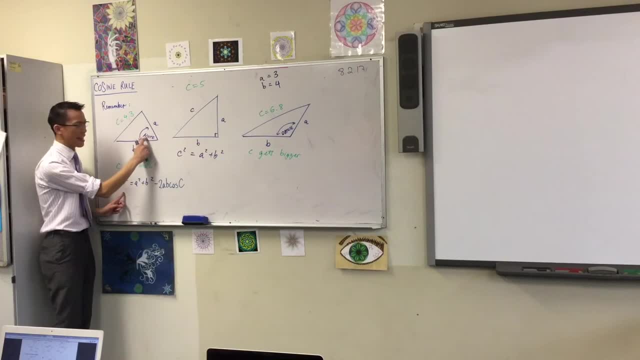 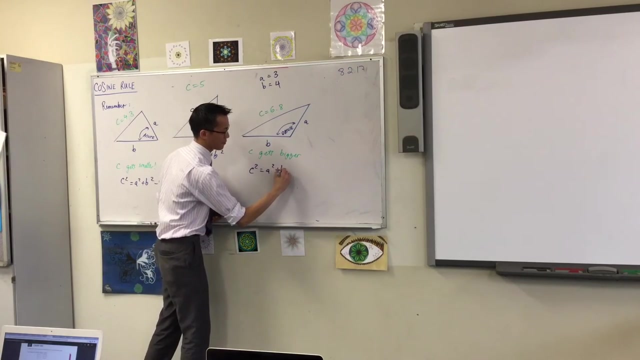 That C must be opposite this C. It's that angle that's in the corner. Okay, People do find symmetry hilarious. Okay, now here's the right thing: different cases. but the cosine rule is so clever that for bigger triangles, you again start with Pythagoras. and cosine does this great thing, even though it. 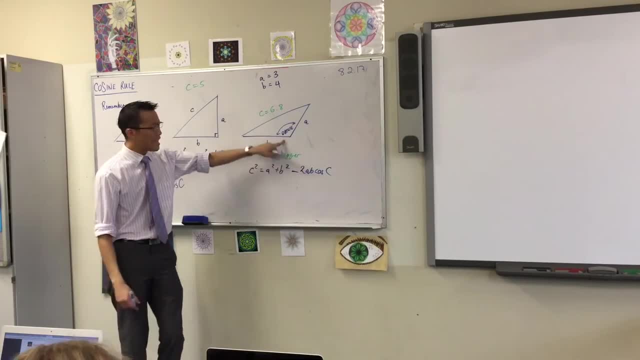 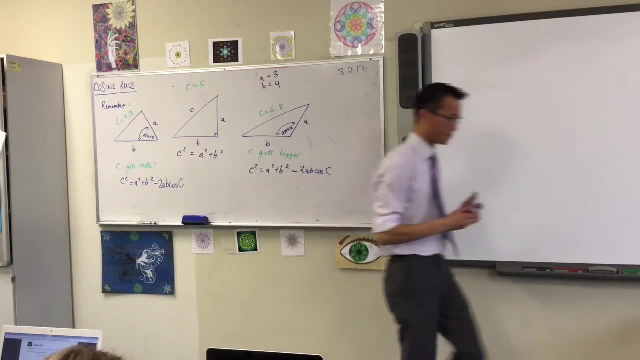 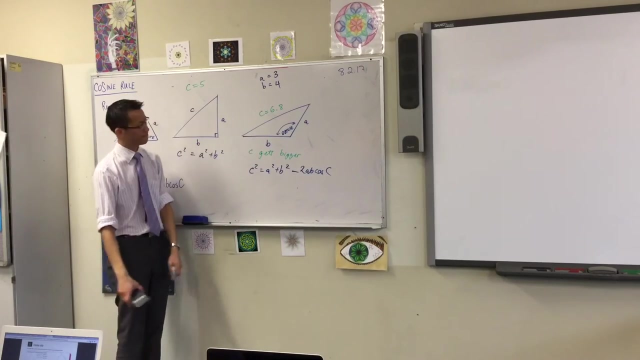 looks like you're subtracting something. if cos is a, sorry, if theta is obtuse or if this angle here is obtuse, actually, once you get your calculator there on my diagram, just for the sake of consistency, what would you call the angle? just give me a rough estimate: 100 degrees, 100 degrees? yeah, let's go with a. 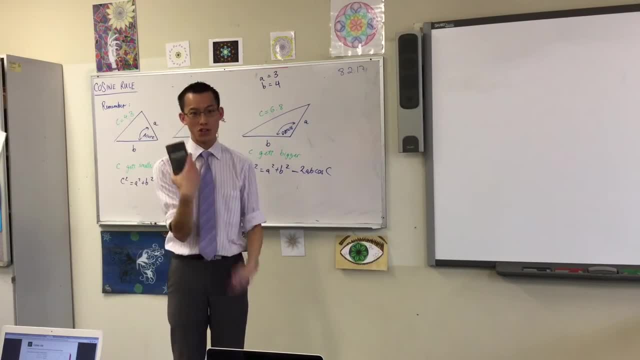 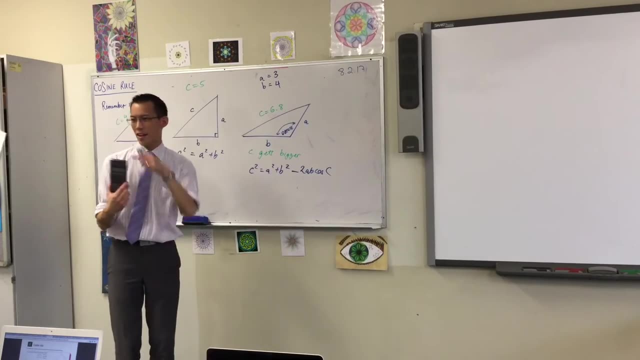 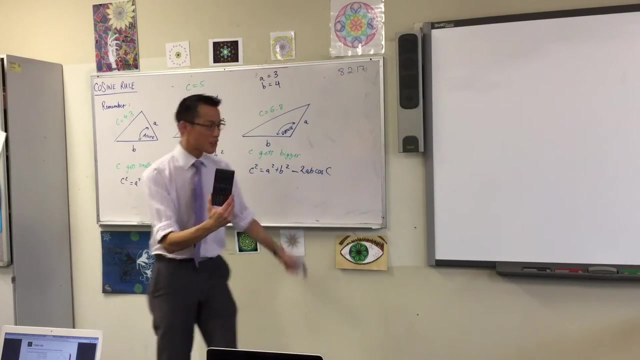 hundred. okay, if it were a hundred, I want you to take your calculator and I want you to punch in cos a hundred degrees, okay. now gives you again a weird string of decimals, but the important thing is right at the front. what do you notice about this number? it's negative. very good. so if this angle is obtuse, cos of. 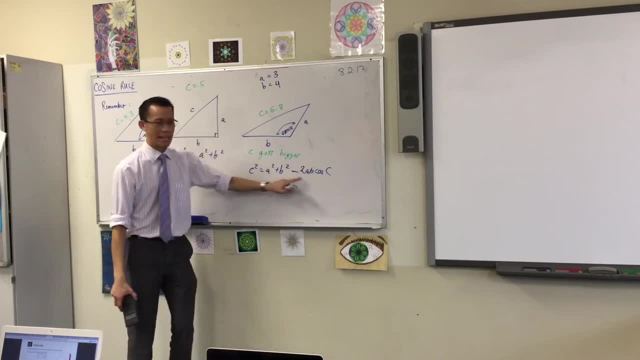 that angle is negative. so if this angle is obtuse, cos of that angle is negative. so if this angle is obtuse, cos of that angle is negative. so if this angle is negative, so if this angle is negative, well, if this guy's negative, what does that mean? it means to cancel out and give you a positive, which it better. 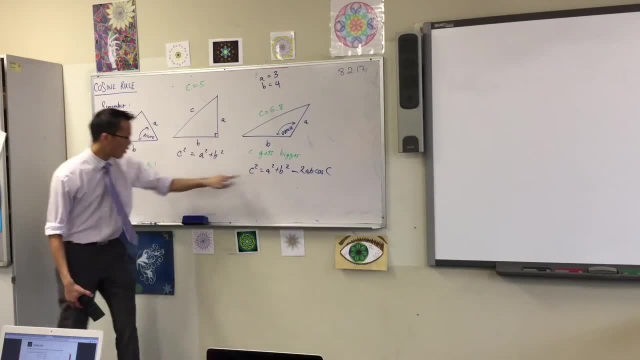 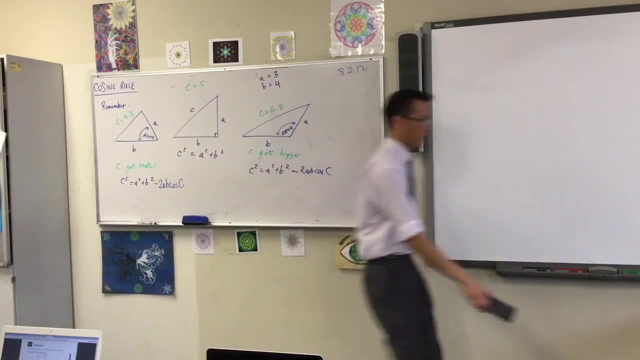 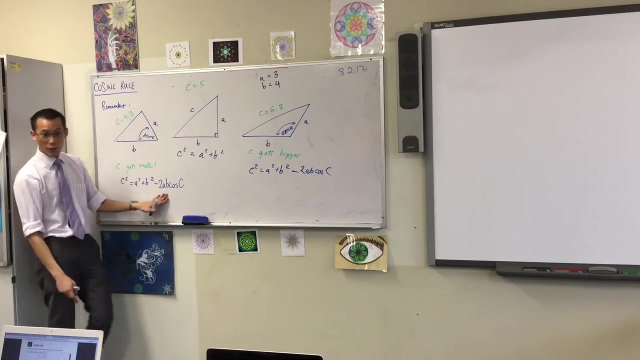 because C gets bigger. you wanted to add. it's one rule. it's the same souped-up version of Pythagoras theorem that works for everything. I've got one more beautiful little thing for you. it just works out. it's the same rule now. same rule here. same rule here. watch this, even if it's.